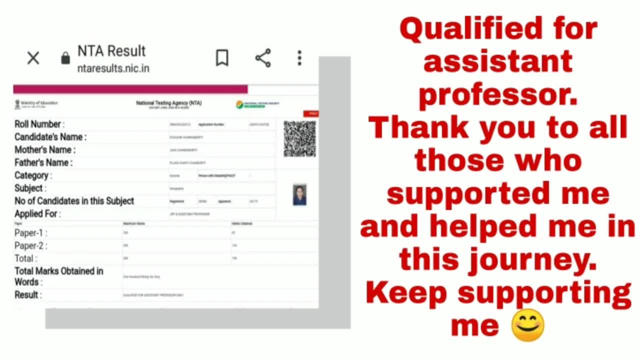 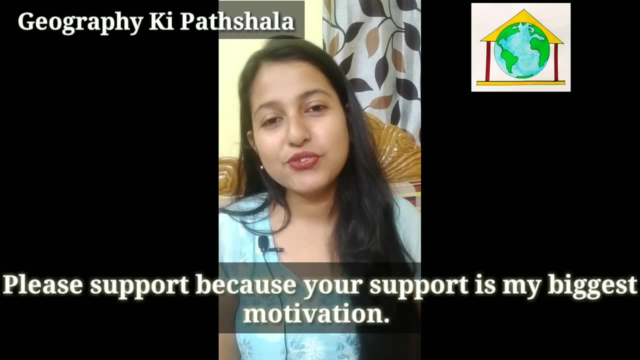 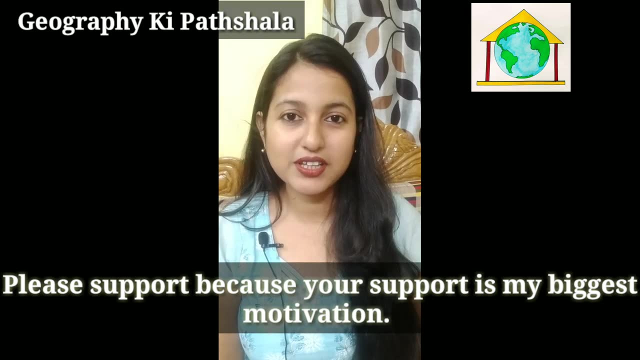 Welcome to all of you in my channel, Geography Ki Patshala. I hope you all are doing well, and in this video class I am going to discuss about the symbols and convectional signs of topo map. and this is the first part of this topic, So let's start with today's video class. 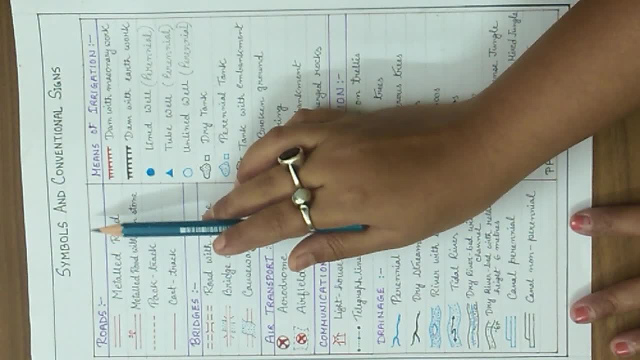 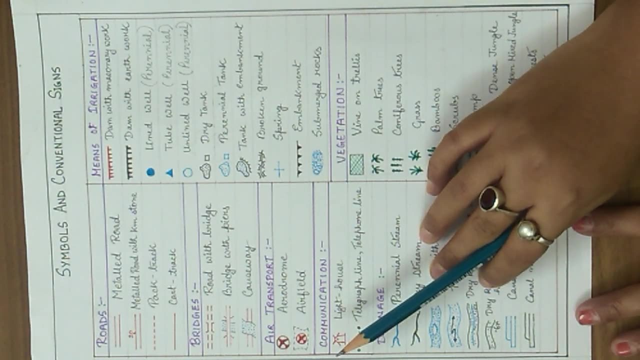 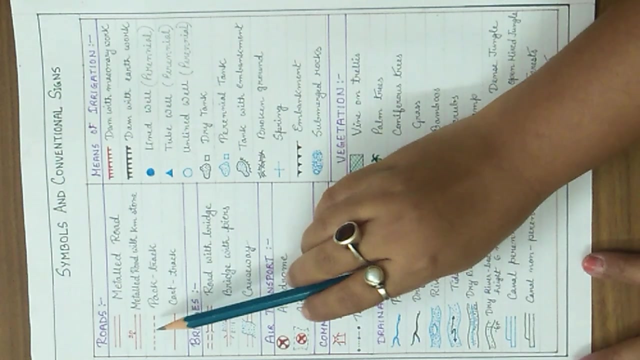 So here you can see that I have mentioned about some symbols and conventional signs which you need to know while doing your topo sheet works. So let's start with some convectional signs of roads. So here you can see that I have mentioned about some symbols. 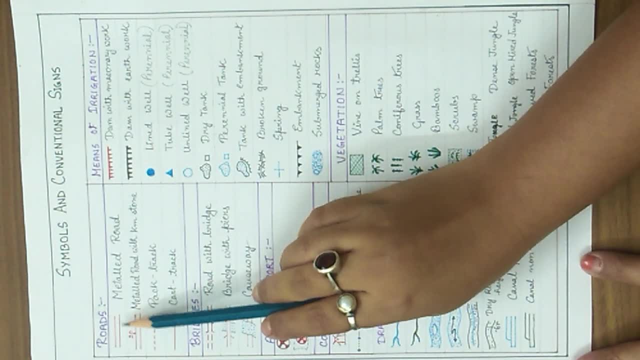 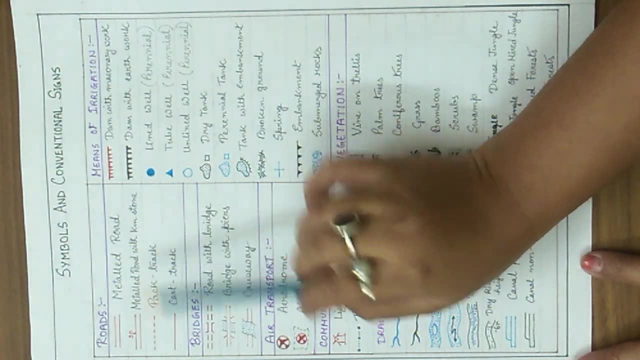 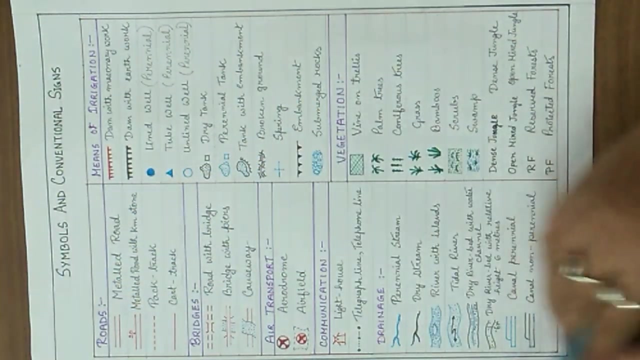 and I have drawn two parallel red lines. So whenever you will see this kind of symbol, that means there is a metal road. Metal road means the pakka road. Especially, you can say that these are kind of national highways or the state highways. Now, if I come to this second one, 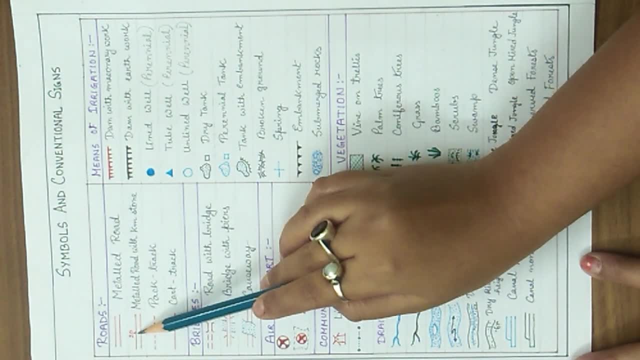 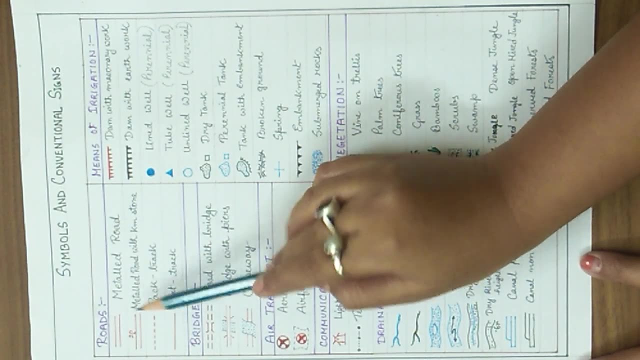 here you can see that I have mentioned about a point and numbered it. So when you will see this kind of symbol, that means it is a metal road with the kilometer stone. See, this is the number and here is the point. So this refers to the kilometer stone. Now, if I come, 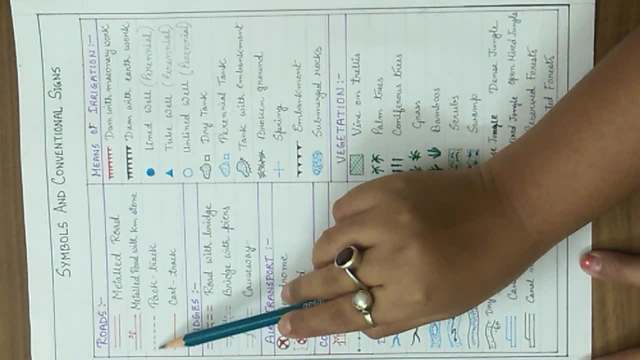 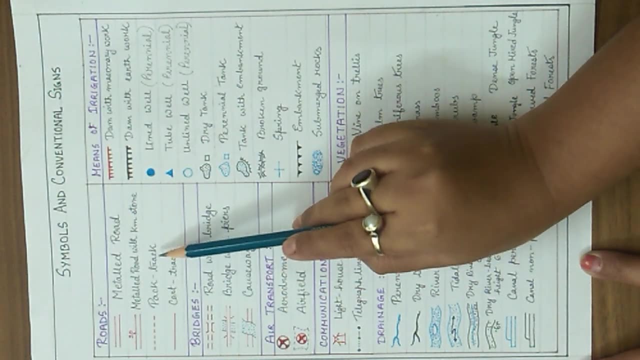 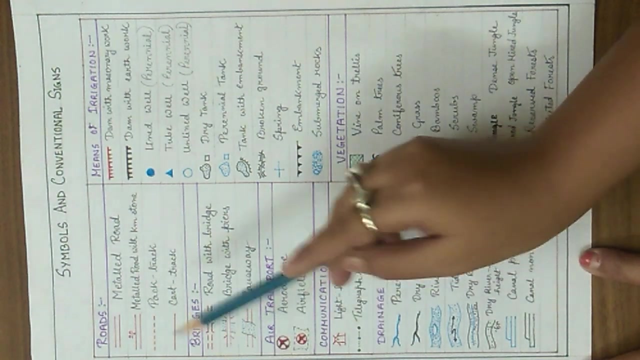 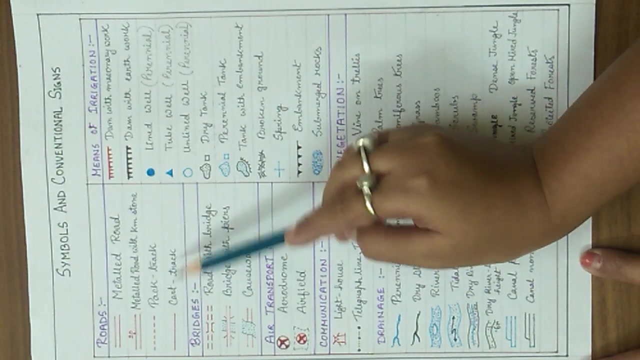 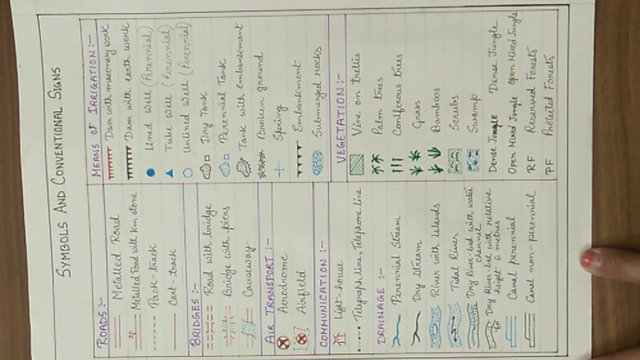 to this next one. this is the red dashed line and this kind of symbol indicates about the pack track. So pack tracks, So these are the tracks of path used either by pack of animals or by group of humans, or maybe by both of them. Now see, here is the single red line. So this indicates about the cart track and it's a rough track, or you can say it's a road over farmland that is unsuitable for ordinary vehicles. 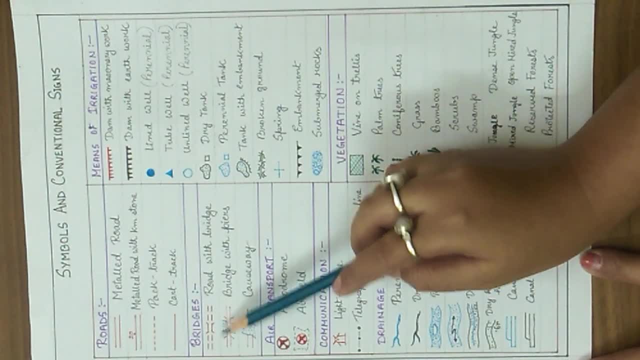 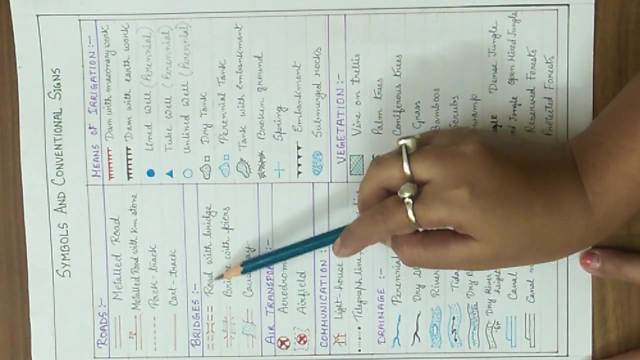 Now next comes about bridges. So these type of symbol- See here I have drawn it's a dashed line and this kind of a symbol is given over here. So this indicates about that: a road with bridge. Next over here you can see that the symbol has changed from the previous one and this kind of symbol over here it indicates about a road with bridge. 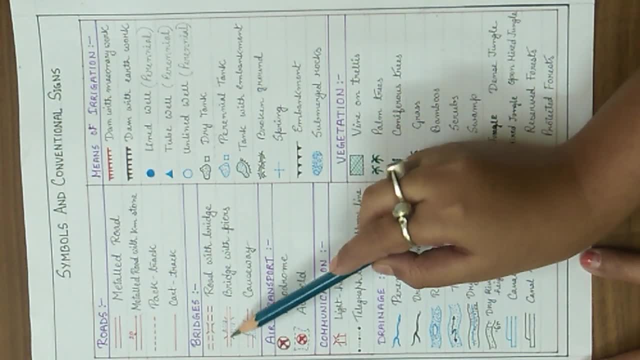